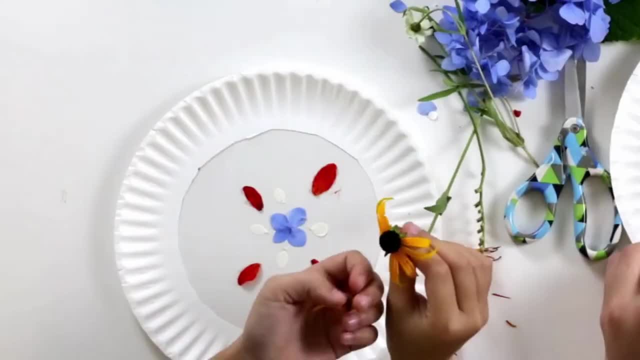 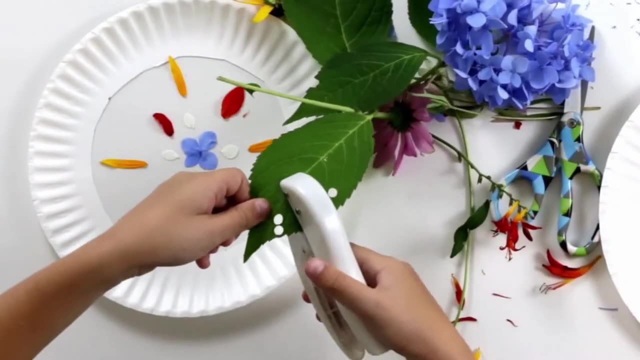 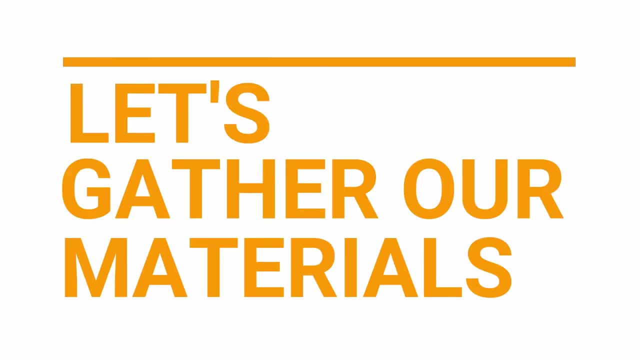 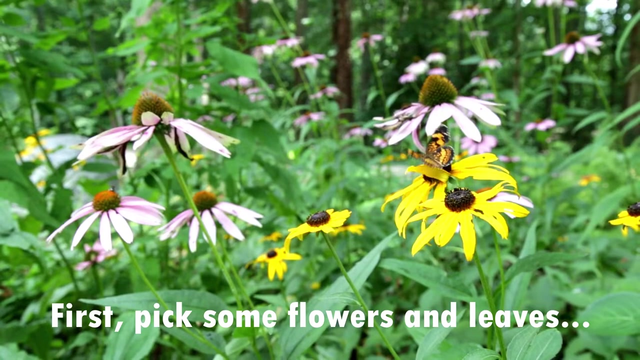 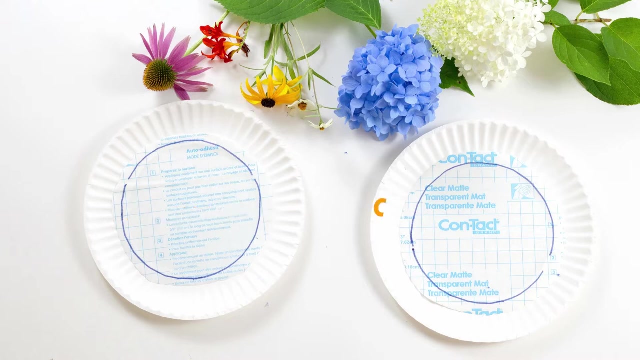 You can make nature sun catchers with flowers, flower petals and leaves- Any colors, any sizes. You can cut larger flower petals and leaves into smaller sizes or tear them. Let's gather our materials, So first pick some flowers and leaves. You'll also need a paper plate, clear contact paper, also called sticky back plastic. 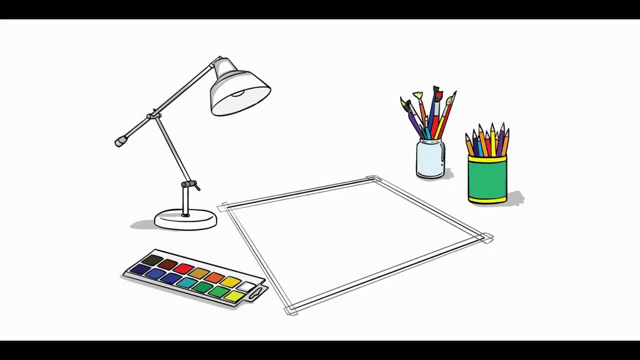 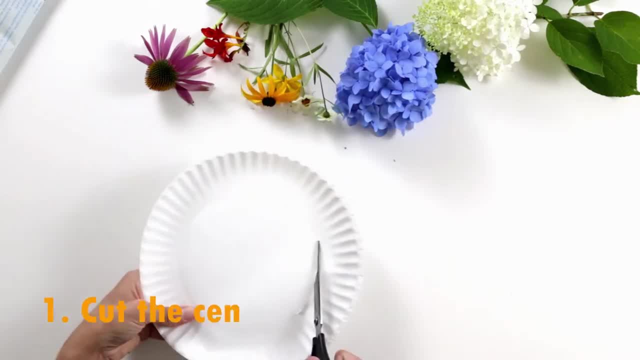 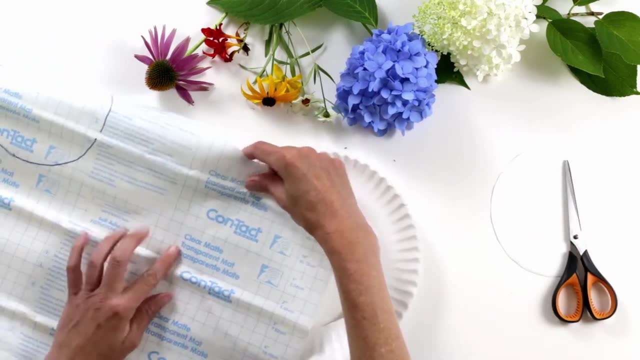 Make the paper plate frame. Making the paper plate frame is a job for an adult or an older child. Ask for help if you need to. To make the paper plate frame, cut the center out of a paper plate. Trace the inside of the paper plate frame onto the transparent contact paper. 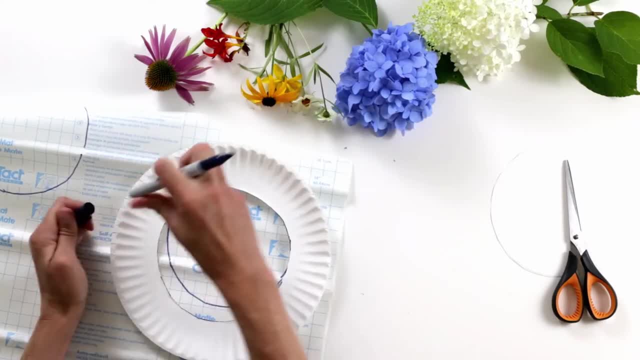 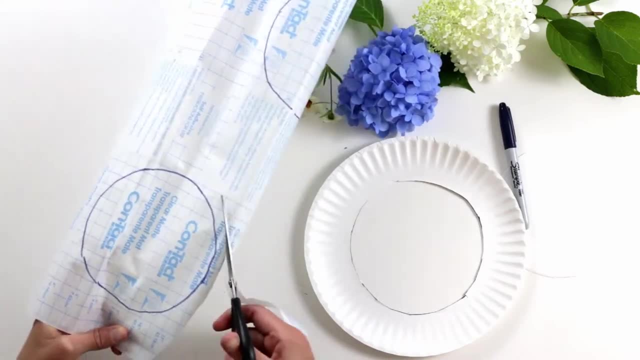 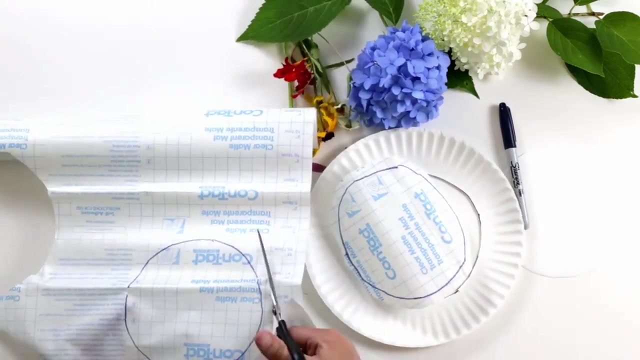 And you'll want to do this twice. You need two circles of transparent contact paper for one frame. After you trace it on with a marker, then cut out those contact paper circles, but cut them out about half an inch to an inch larger than the circle you drew. 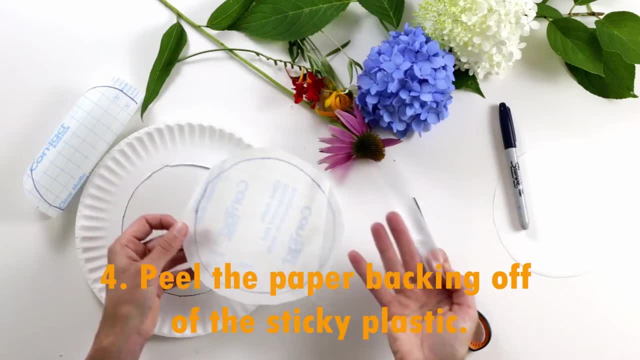 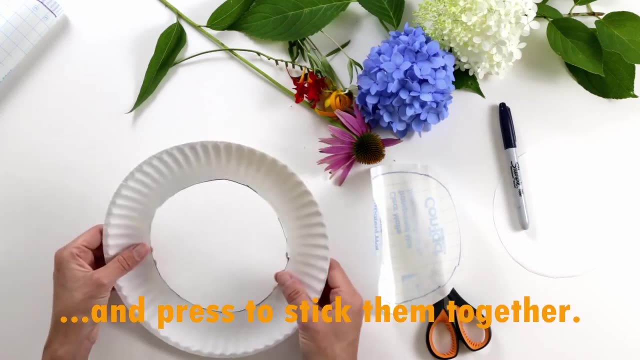 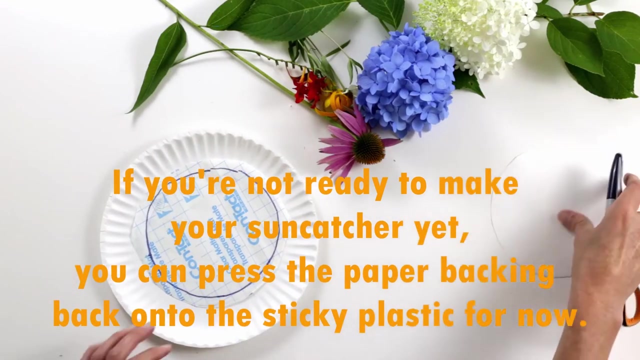 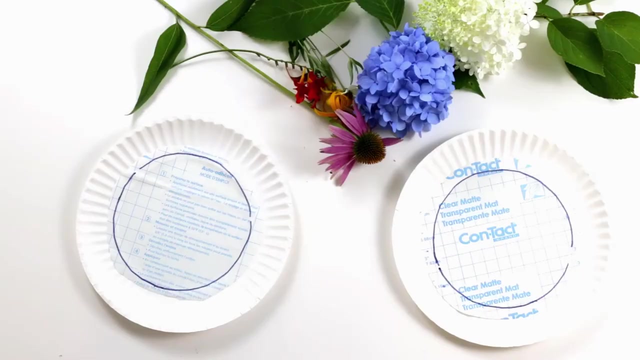 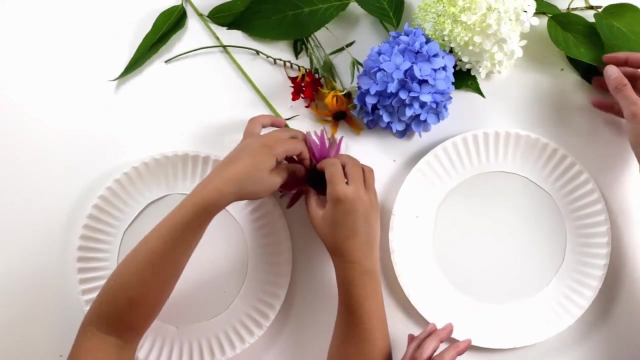 Now what you'll do is peel the paper backing off of the sticky plastic and lay it on the table, sticky side up, Center the paper plate over the plastic and press it to stick them together. Let's create. Now it is time to take flower petals and leaves and press them to the sticky contact paper. 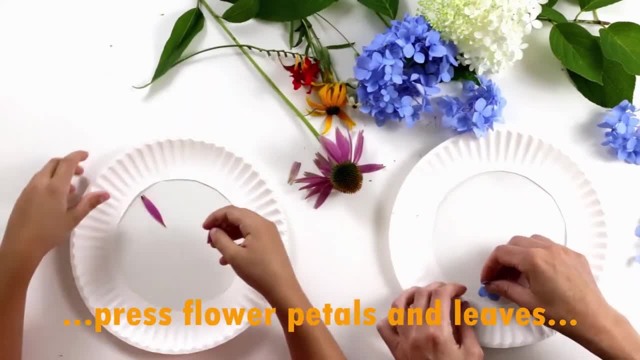 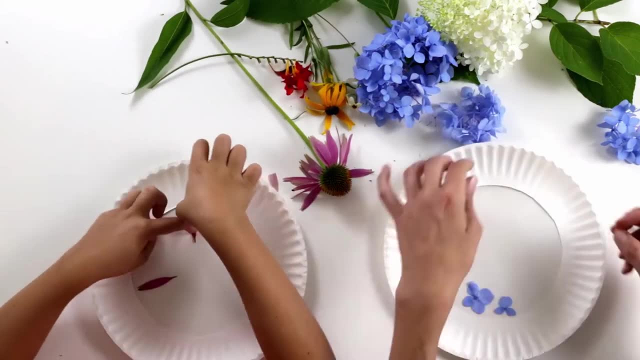 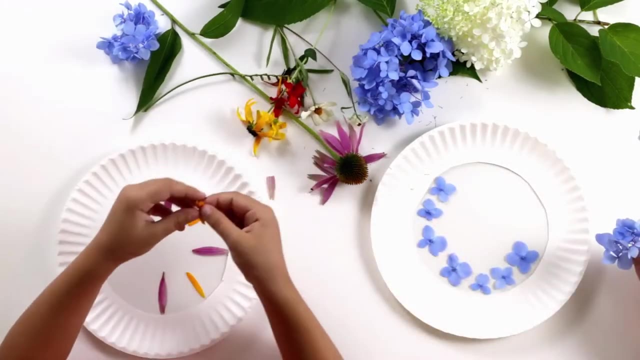 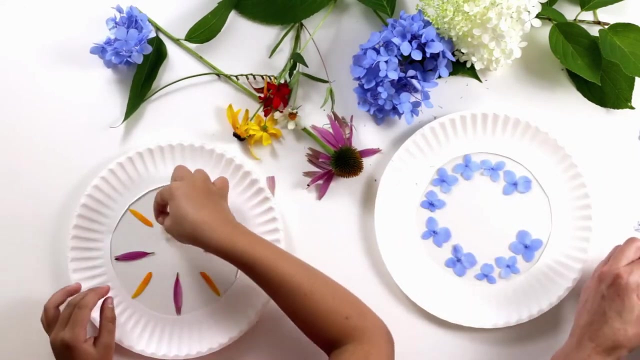 You can do this in any design you like. You can do it abstractly, or you can make pictures or patterns or mandalas. You can make faces or butterflies. We've done a lot of different things. If a flower is large or bulky, you can pull off individual petals. 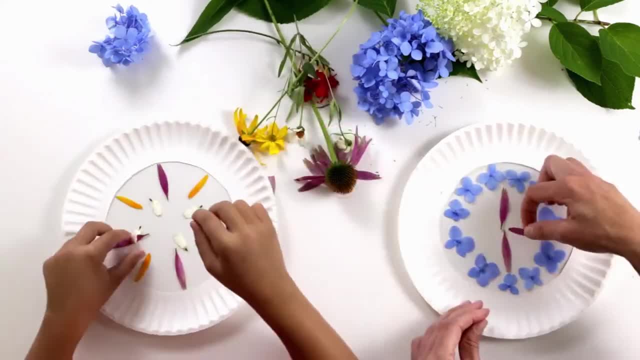 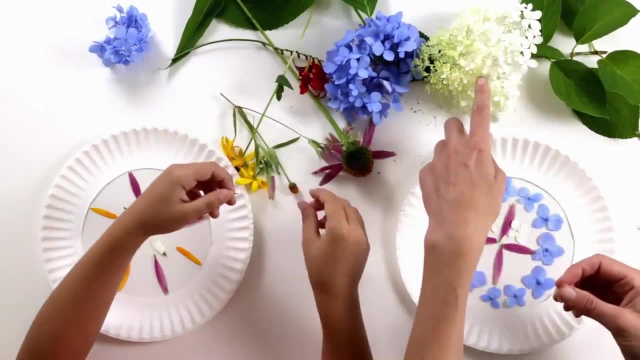 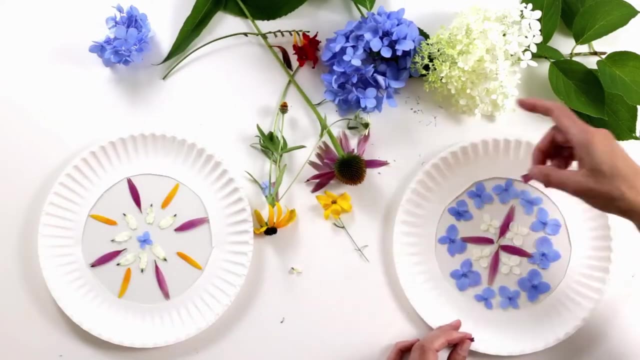 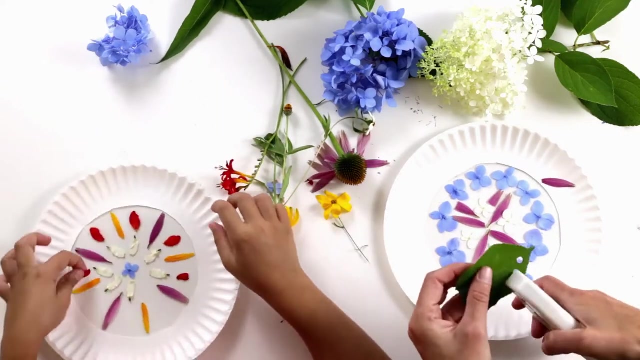 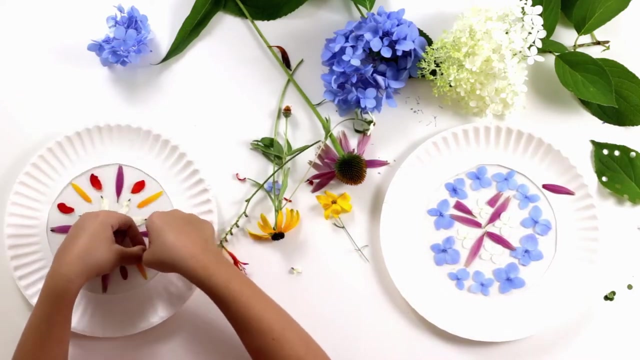 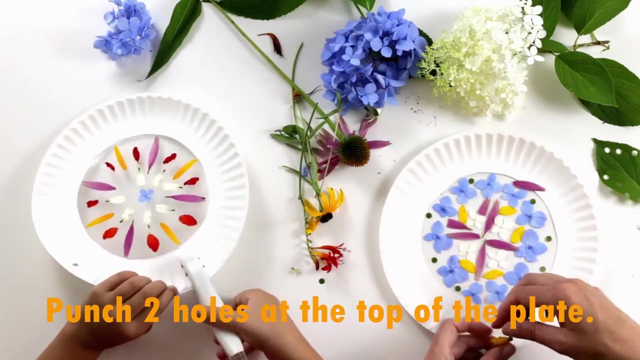 And even tear petals into smaller pieces, Or you can use scissors to cut them into smaller pieces And, if you like, you can use a hole punch to punch small holes out of leaves or flowers. When you're finished with your sun catcher, you can add a hanging handle by punching two holes with the hole punch at the top of your paper plate. 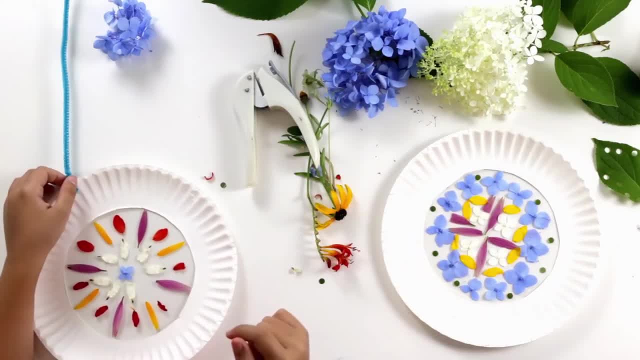 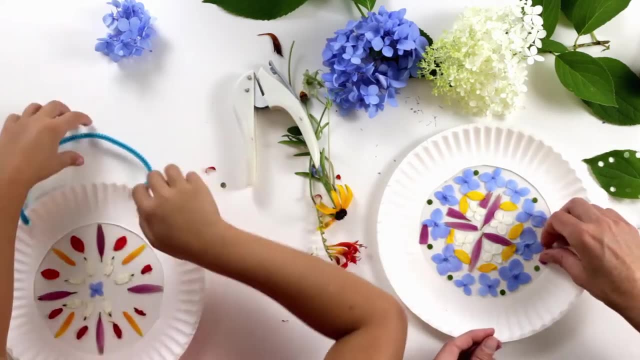 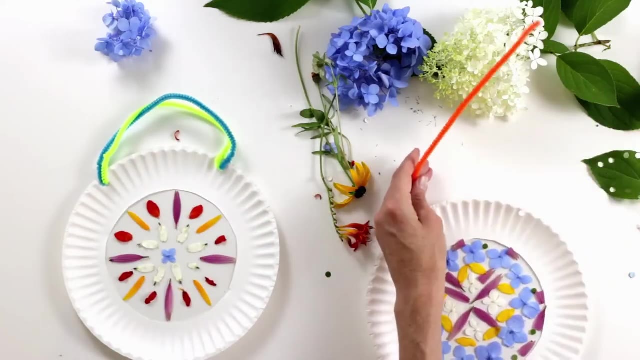 And then threading a pipe cleaner through each of those holes. Bend the pipe cleaner over and twist it around itself to secure it in place, And this will provide a hanging handle or a carry handle for your sun catcher. Now get your second contact paper circle and remove the paper backing. 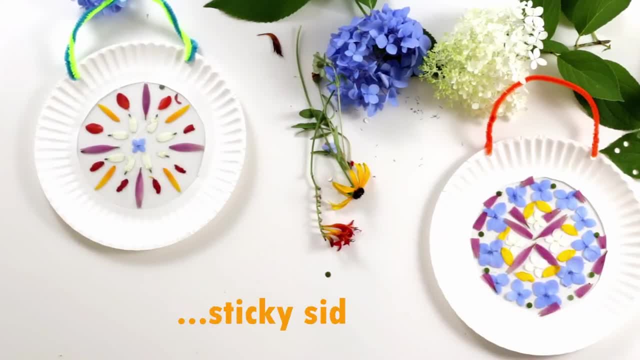 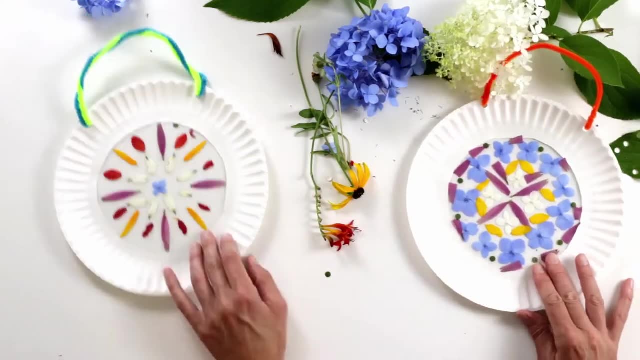 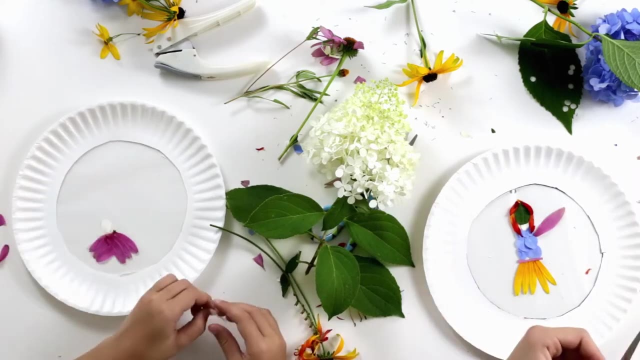 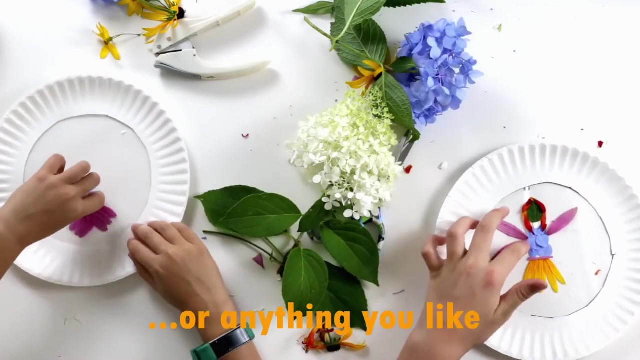 And then press it over your flower design sticky side down. You're basically creating a flower sandwich between the two pieces of transparent contact paper. This helps protect the flower design and also helps preserve it for longer, And you can also decorate the paper plate frame. 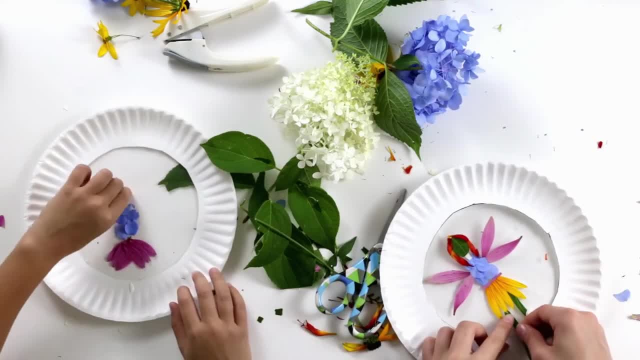 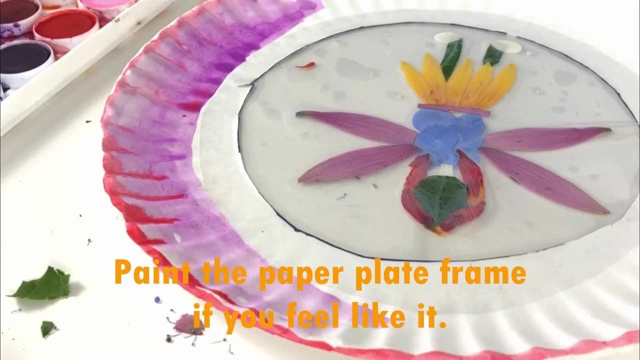 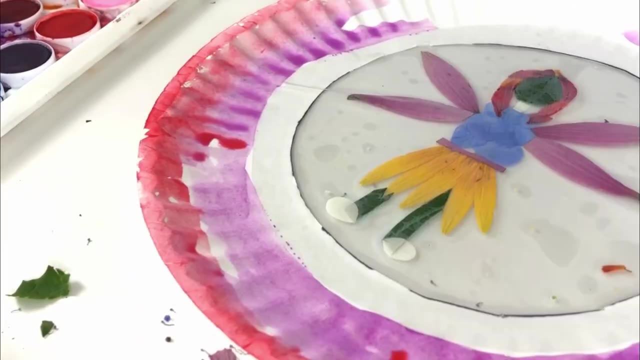 You can paint it with watercolors or any other color you like, And you can also decorate the paper plate frame. And you can also decorate the paper plate frame. You can paint it with watercolors or any other color you like, Or decorate it with markers or anything you like. 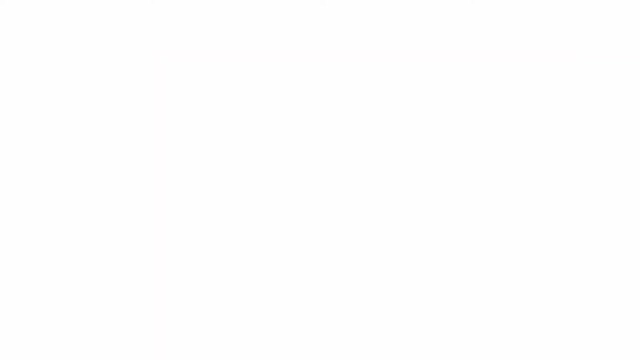 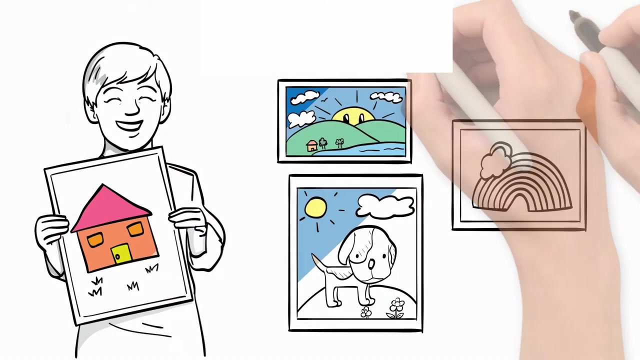 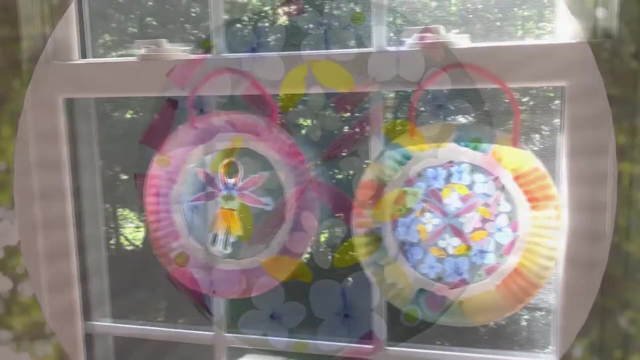 I hope you enjoyed this art activity. These flower petal sun catchers will not last forever. They will not hold their color forever. The flowers and leaves are parts of nature, ephemeral. They will begin to decay And that's totally fine. 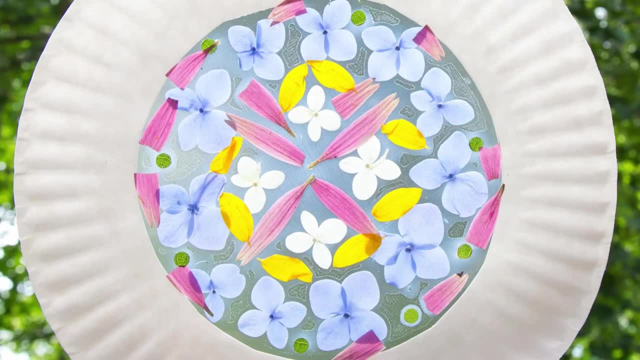 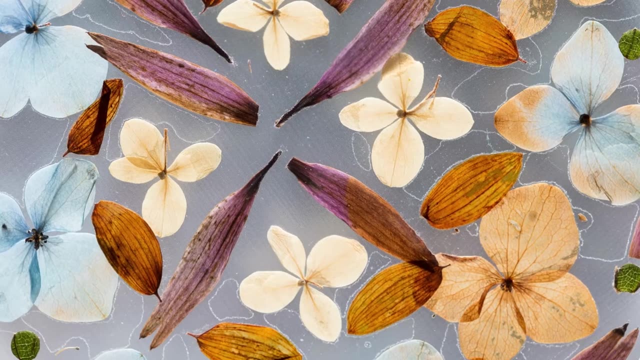 It's a really interesting process to watch And they're still beautiful after that happens, And just keep them up as long as you like And then create a fresh one anytime you like. It's time to create. It's time to create. 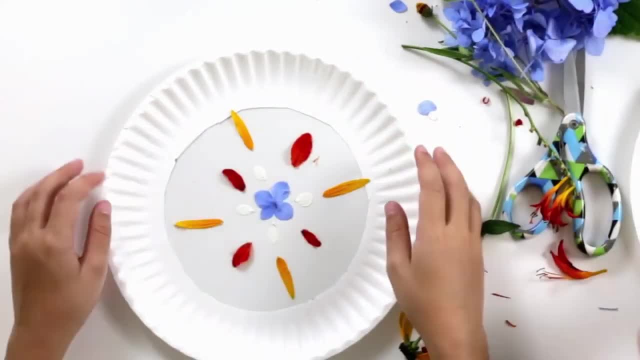 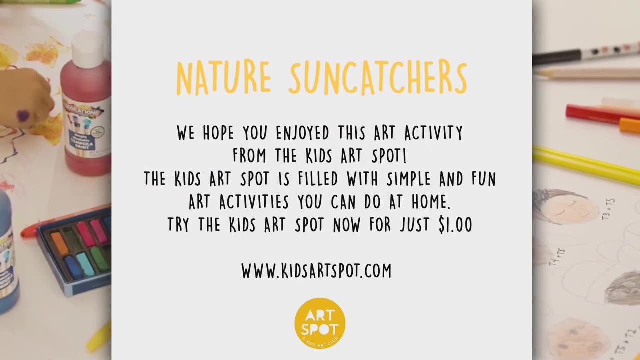 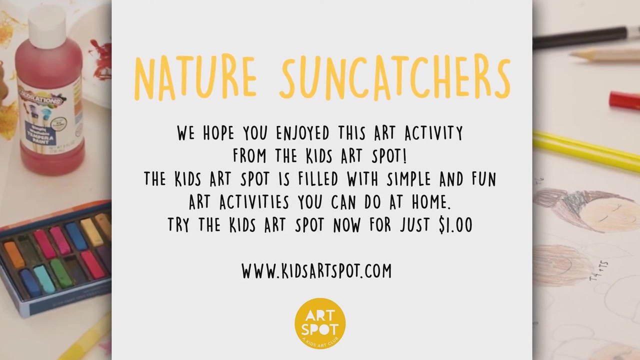 It's time to experiment and make something great. Let's explore the magic of art. We've all been created from the very start. Show your own color In your own way. It's time to create. It's time to create. 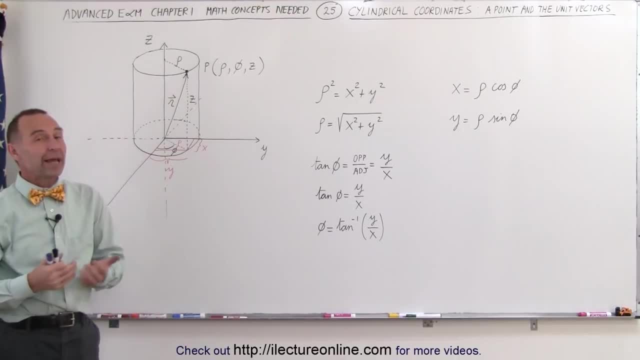 Welcome to ElectronLine. With electricity and magnetism it's often more convenient to express things in cylindrical coordinates instead of Cartesian coordinates, And later on we'll see that sometimes it's even better to use spherical coordinates. But first let's concentrate on 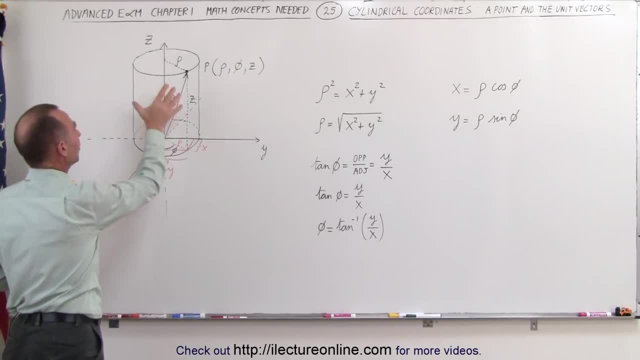 cylindrical coordinates, And you can see that I've drawn a cylinder here about the XYZ coordinate system, And notice that whenever we're dealing with objects that look like cylinders, cylindrical coordinates are often the best thing to use. Let's pick an arbitrary point in space, So I have. 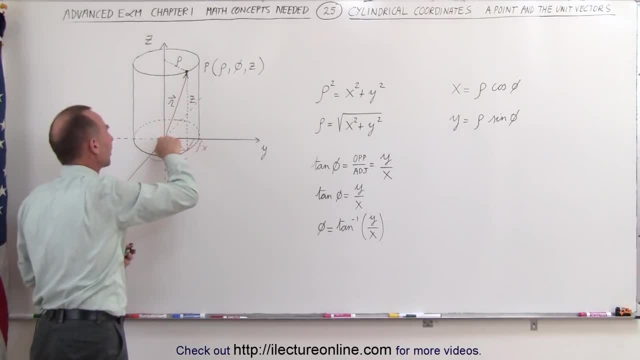 the origin. right here, I draw my unit vector- not my unit vector, but my position vector- to this point, right there, And that's the point of concern. Notice the three variables that we have. We have rho, phi and z. What do they mean? Well, rho represents the distance from the z-axis to the 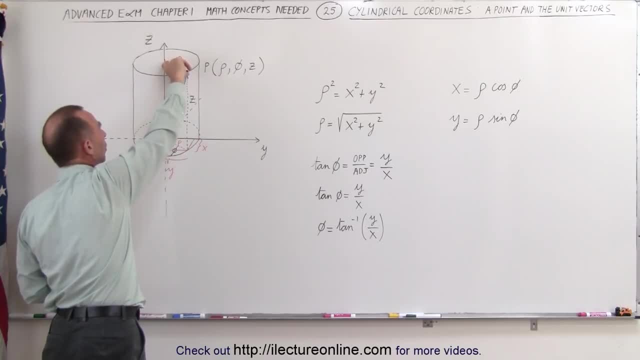 point. So from here to here, that distance here is rho. Notice, when I project that onto the XY plane I have the rho down here as well. So that's simply the distance from the z-axis to the point in space. Phi is an angle that references from the 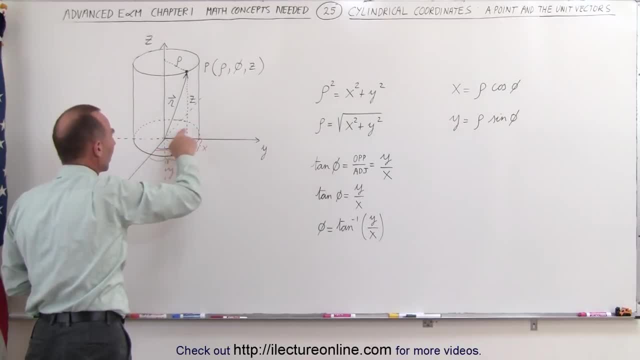 x-axis towards the y-axis and on around like this. So if I go around in this circle, starting from the x-axis, when I draw a line from the z-axis to the point P, how big of an angle is that from the x-axis to the line that goes from zero to the point? 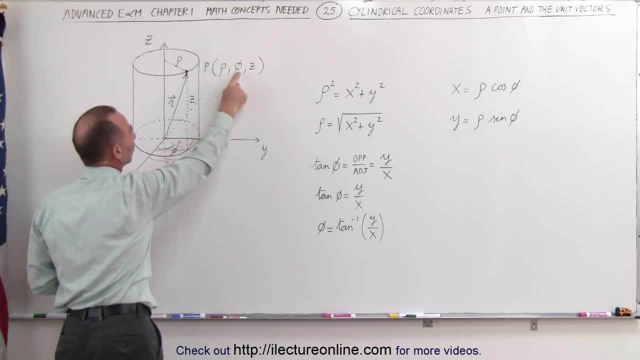 Well, the z-axis is the distance from the z-axis to the point P. So that's the distance from the z-axis to the point P. And finally, the third coordinate, z, is the distance from the XY plane in the vertical direction to the point of.